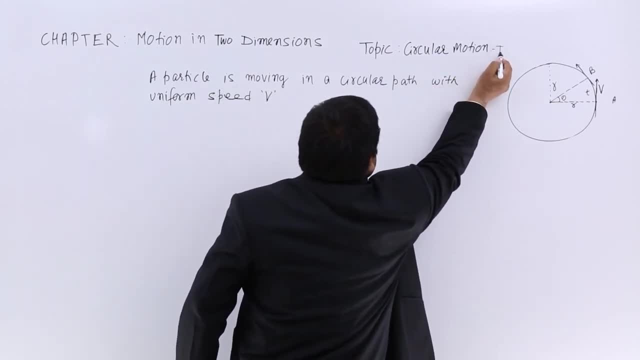 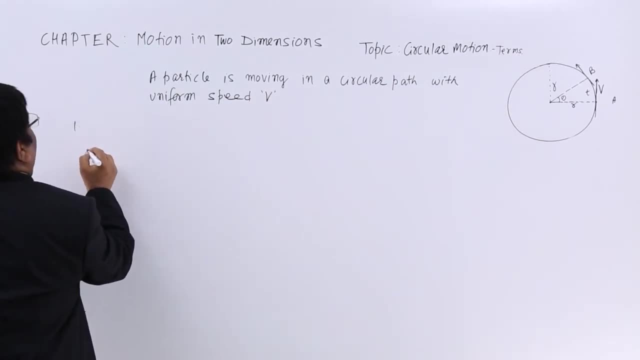 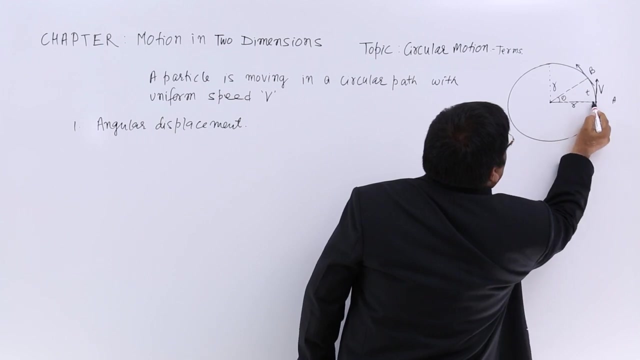 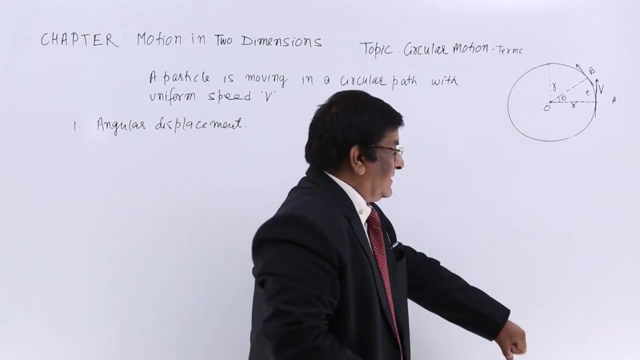 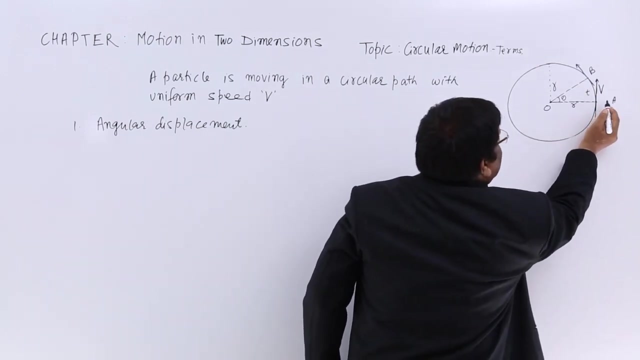 different terms related to this terms. Number 1 is angular displacement. This is a radius- we can treat it as a rod- which is fixed at this point o and this keeps on moving like this. At any point we start our clock. at that time this radius was here, then the time keep on. 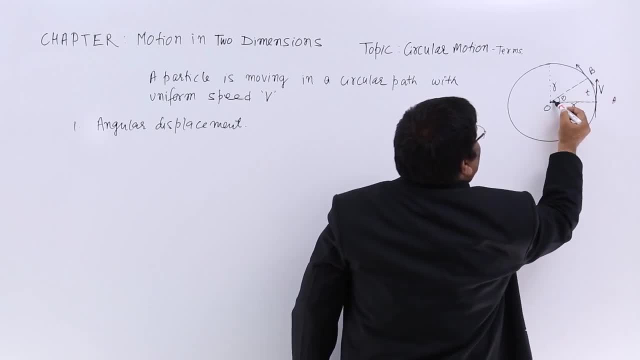 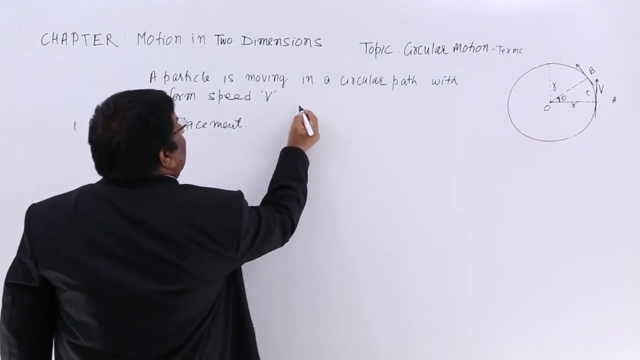 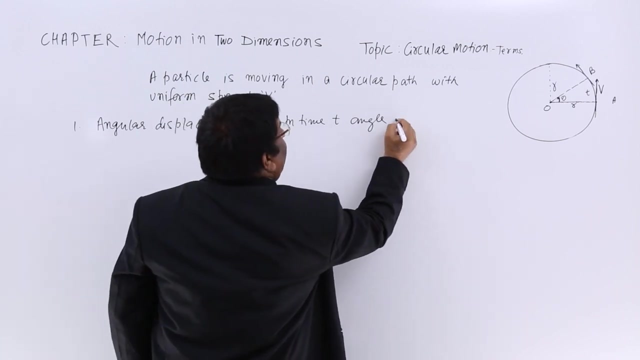 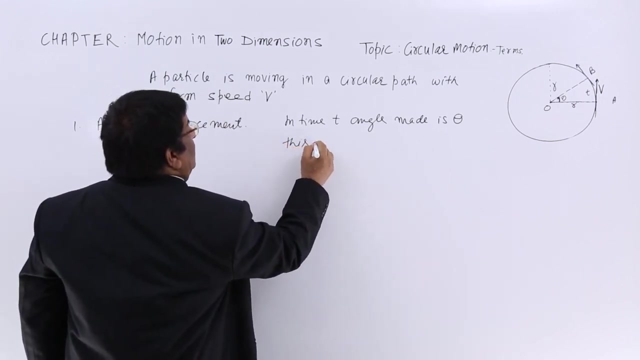 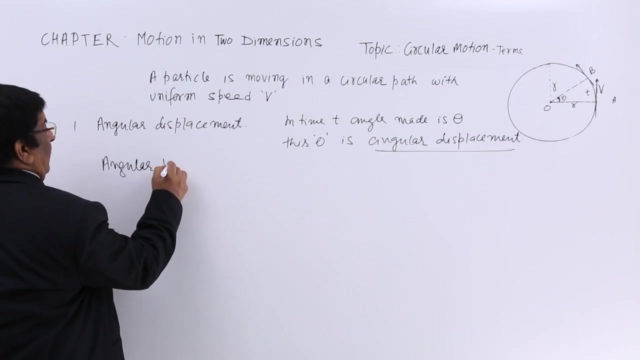 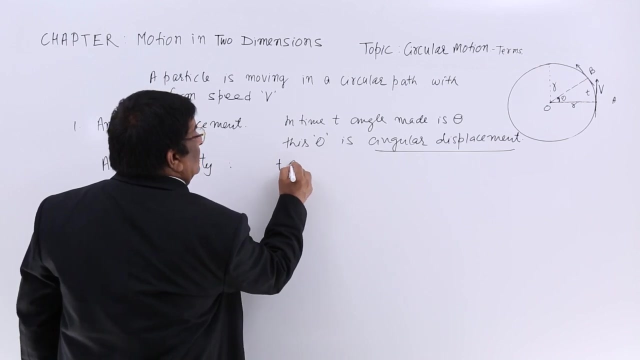 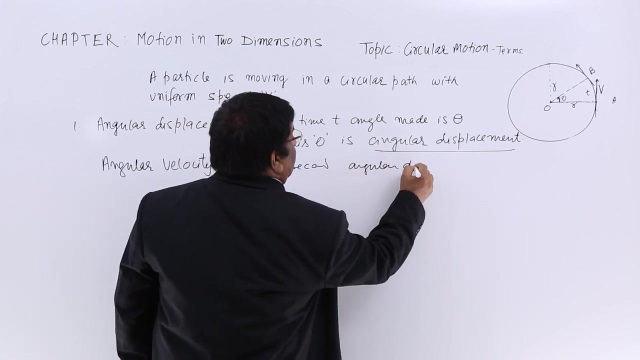 passing, after time t has passed, it has reached this position and this angle made is theta. So in time t angle made is theta. This theta is called angular displacement, that is number 1.. Now angular velocity In t, second angular displacement. angular displacement is theta. 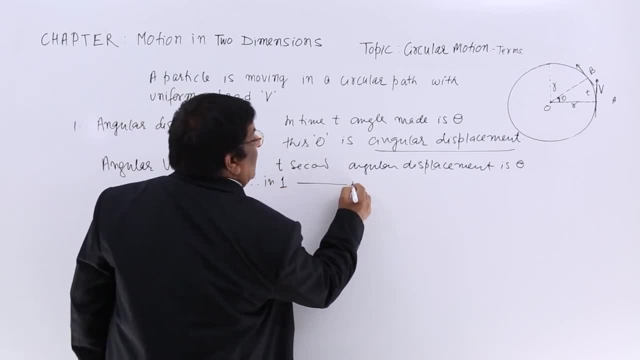 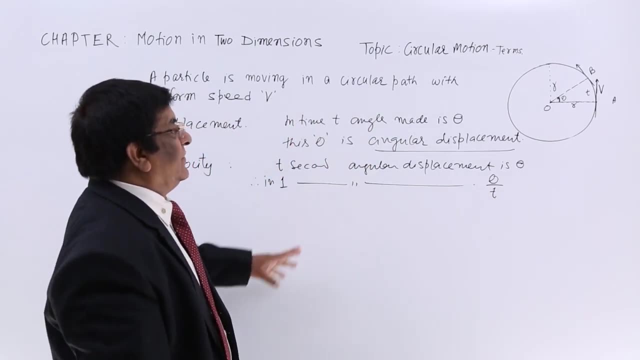 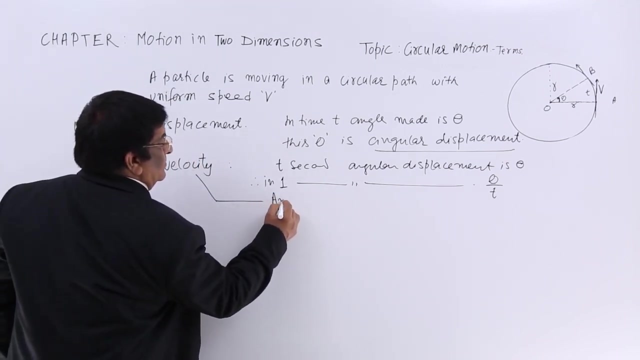 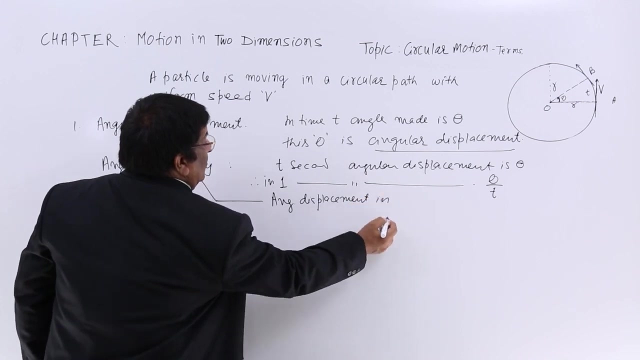 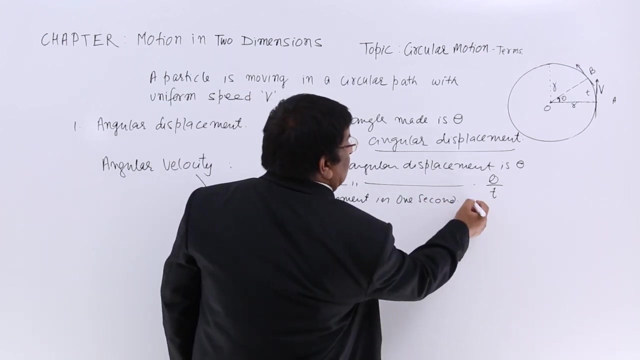 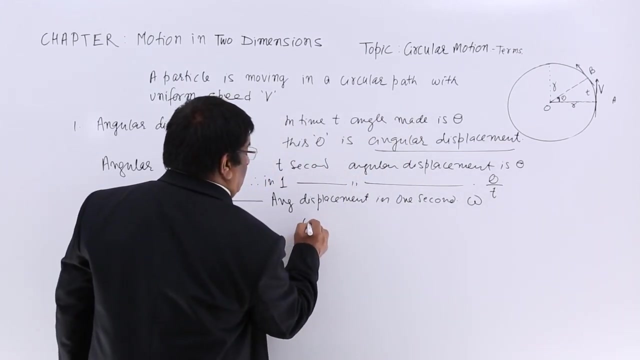 Therefore, in 1 second the angular displacement is theta upon t. This is called angular velocity, that is, displacement in 1 second, angular displacement in 1 second, Thank you. and we give it a symbol, omega. So we have the equation: omega is equal to theta upon 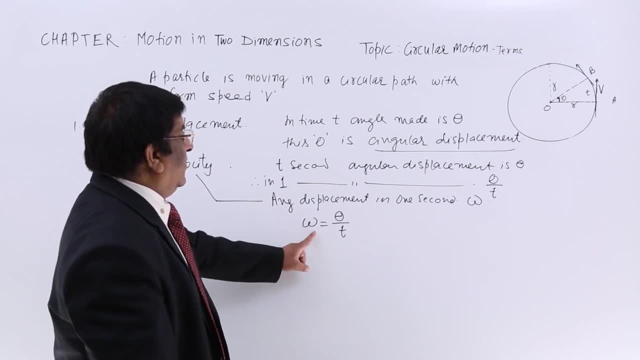 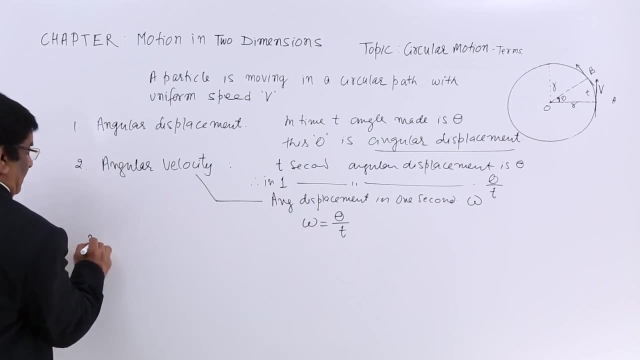 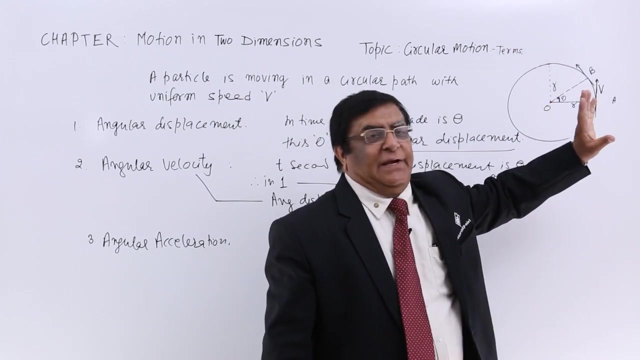 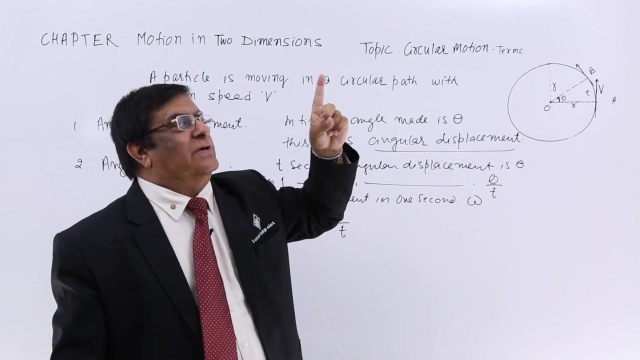 t. This is the relation of angular velocity. Then is angular acceleration. Suppose it is not moving with angular, it is not moving with the uniform speed and it increase its speed. How? When you switch on a fan, initially it runs slow For 360 degrees. it takes 5 seconds. 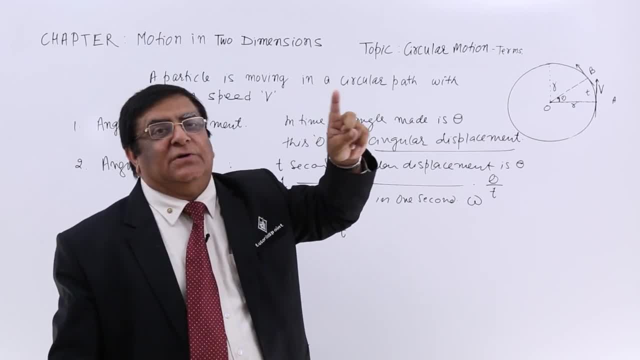 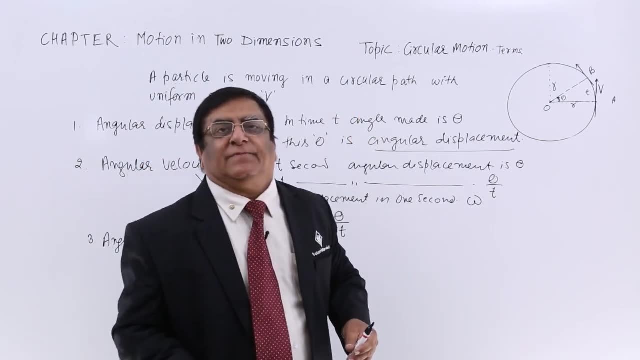 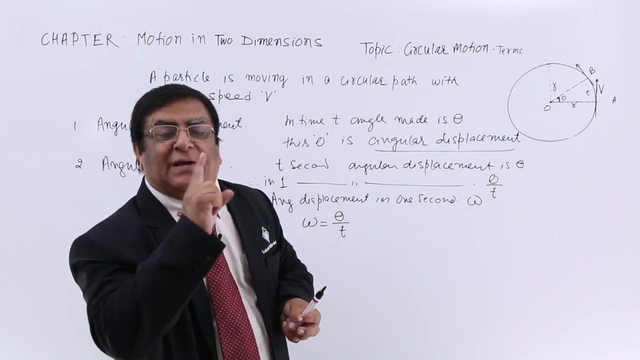 then it becomes fast. For one round it completes in 4 seconds, then in 2 seconds, then in 1 second and it becomes very fast. What is happening? We say this is example of angular acceleration: The angular speed which was 60 degree in 1 second. now it is. 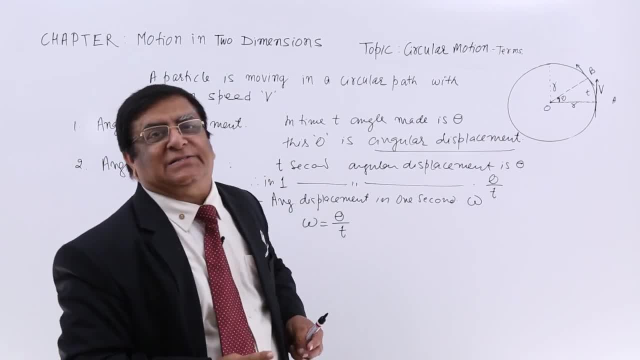 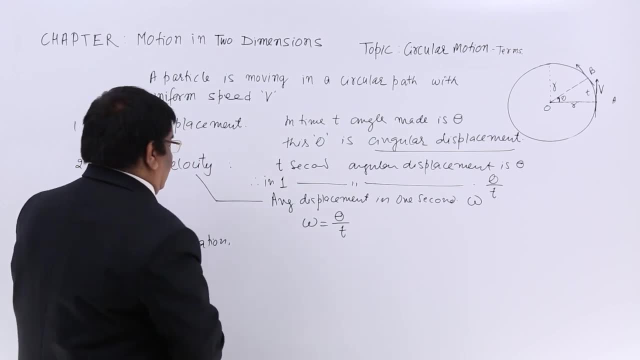 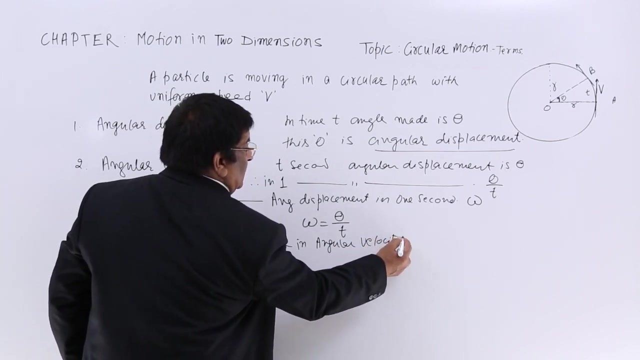 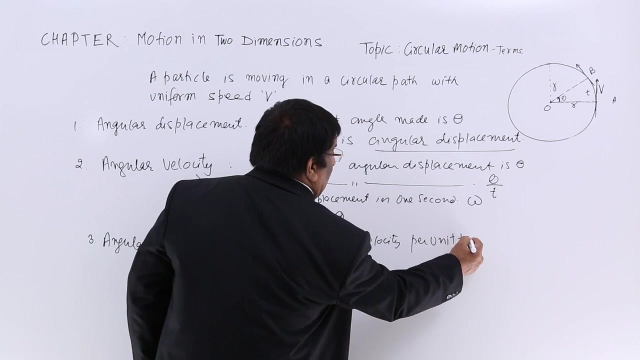 120 degree in 1 second, then it is 180 degree in 1 second. So angular speed is increasing. that is acceleration. How do we calculate it? Angular acceleration: first, define change in angular velocity. This is definition: change in angular velocity per unit time and with. 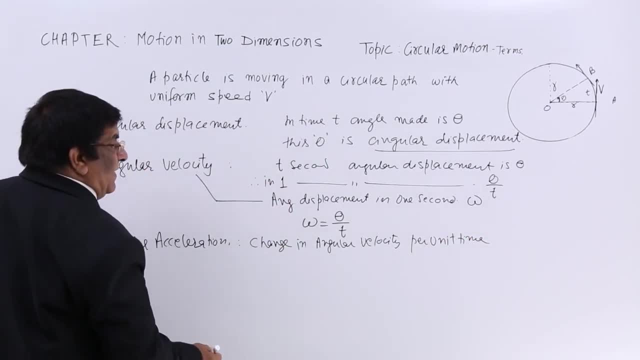 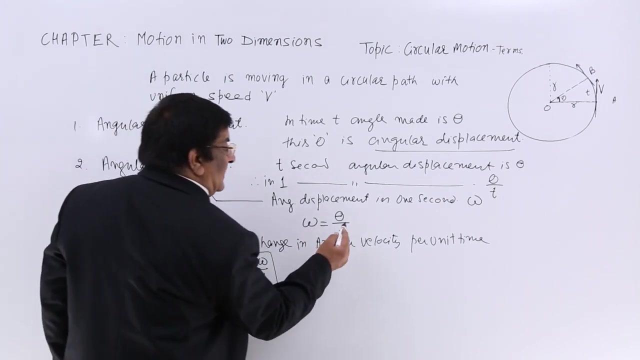 this definition we make the equation that angular acceleration A is equal to- sometimes we write it A some time. alpha is equal to rate of change of angular velocity, d, omega by dt. So this is angular acceleration. This we can write at this or instantaneous value of angular velocity is: 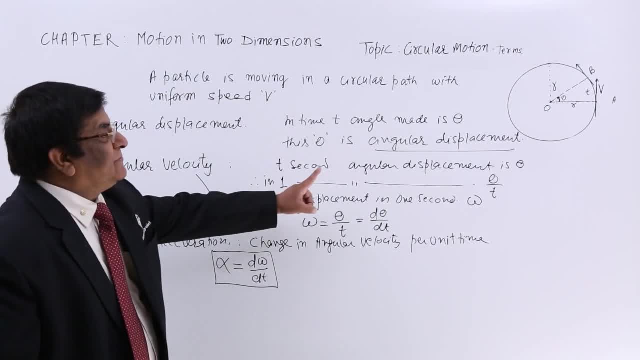 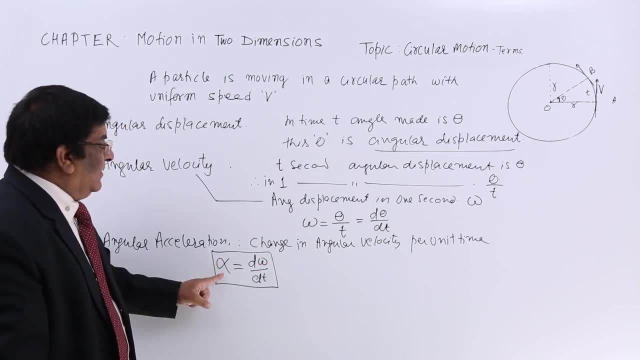 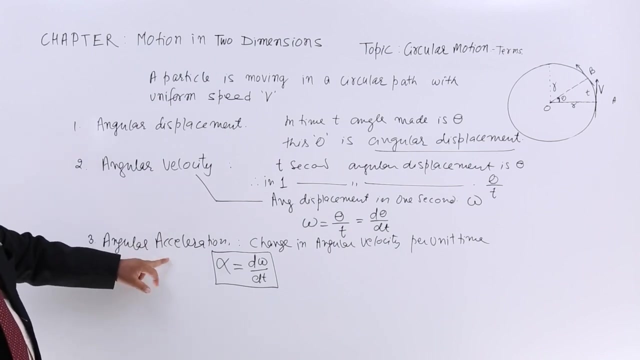 d theta by dt. So displacement, angular displacement theta, angular velocity, d theta by dt, omega angular acceleration is d omega by dt. So these are displacement velocity and acceleration. because we are measuring it with help of angle, we call them angular, angular, angular. This 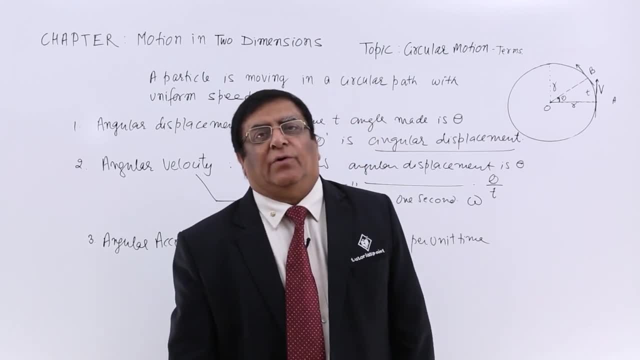 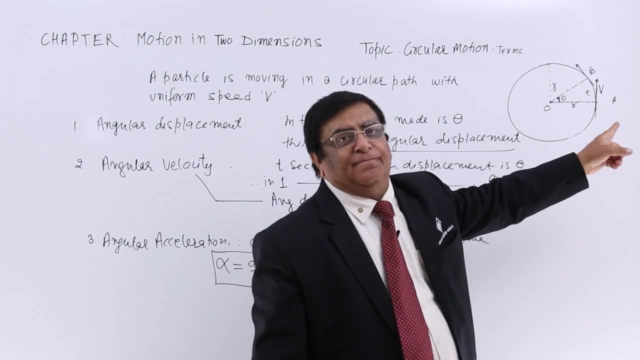 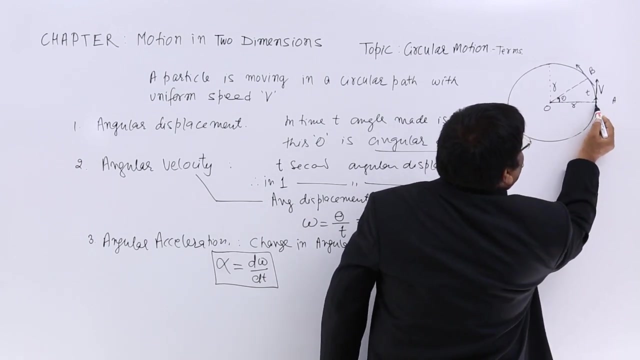 is happening in a circular motion. Now at the end of this… Yes, Now at the end of this… Ah… arm. this is the point A, which keeps on moving at different position If I take the speed of this in this direction. this, this is a line line. If it is a line, its motion will. 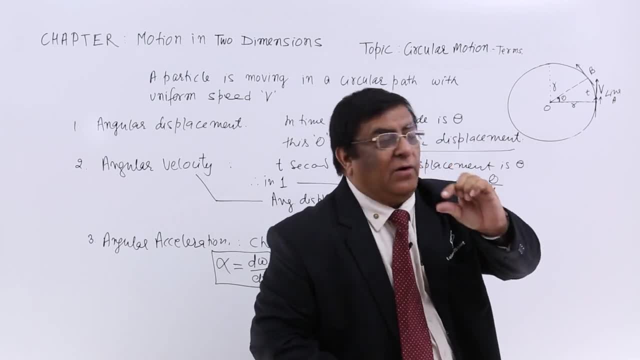 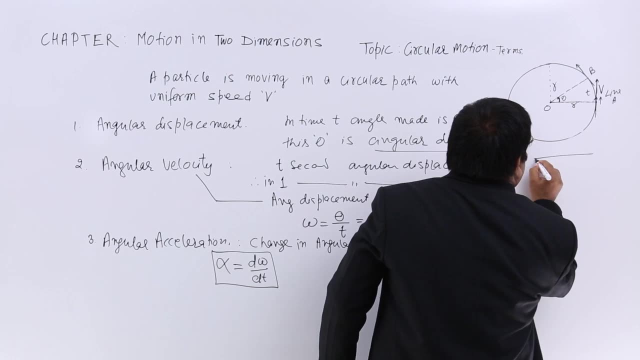 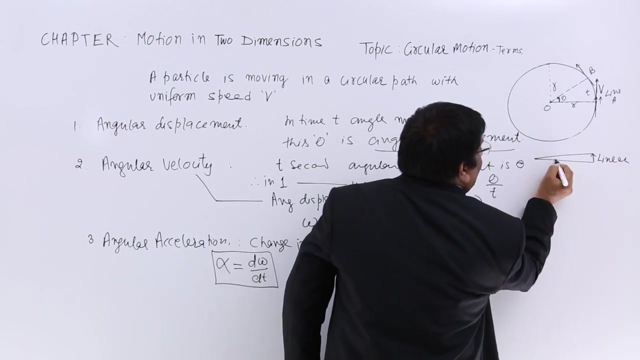 be linear motion For a very small, for a very small part. we see that linear motion is taking place here. linear And angular is taking place here, angular, And this is r theta. okay, Suppose, from point this to this there is a small distance, x. So this is what x represent. 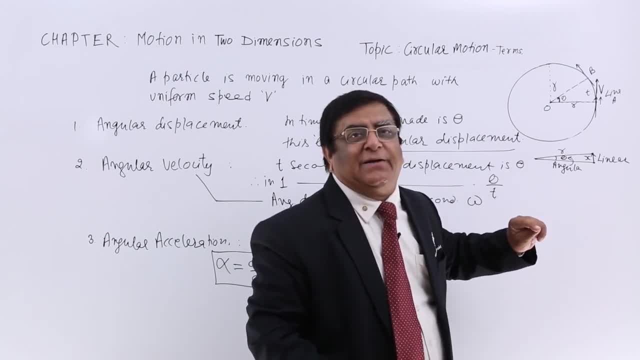 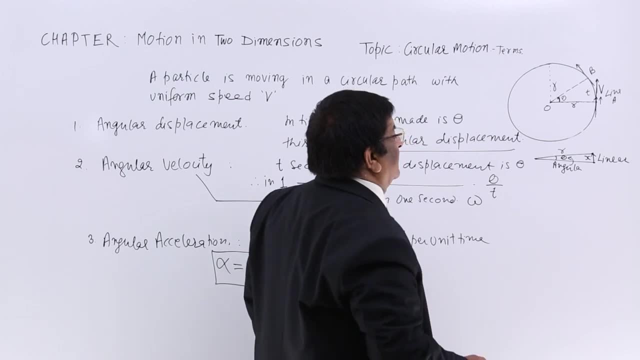 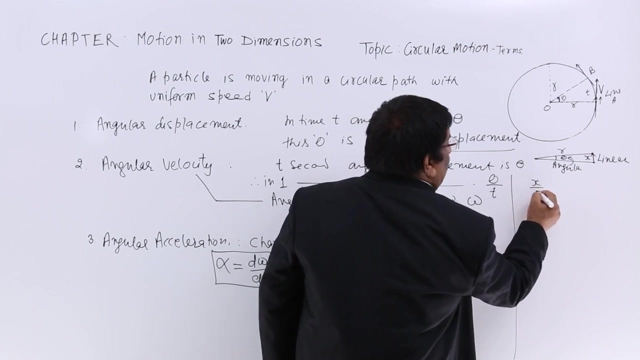 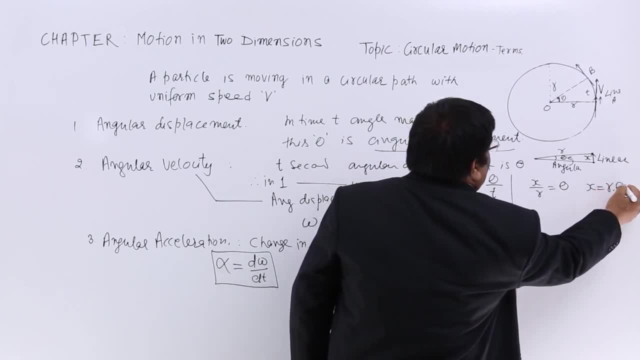 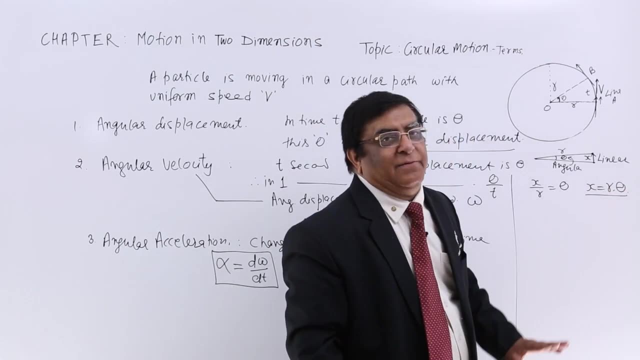 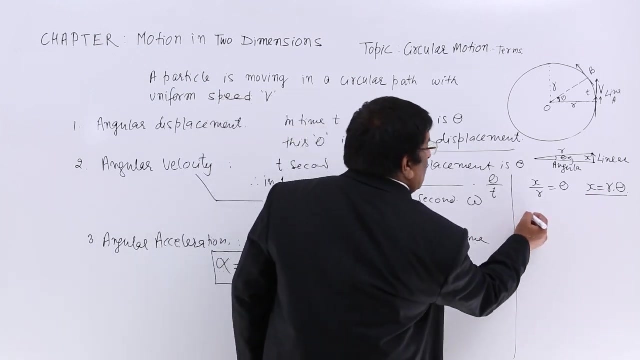 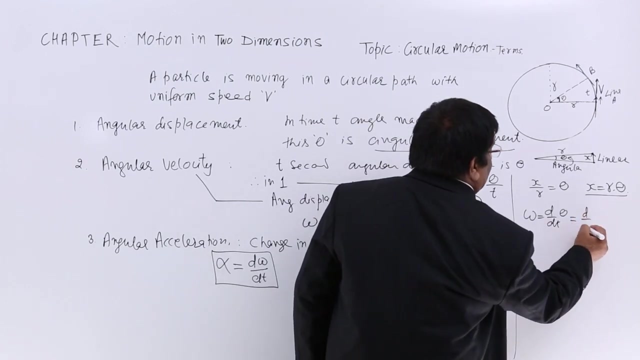 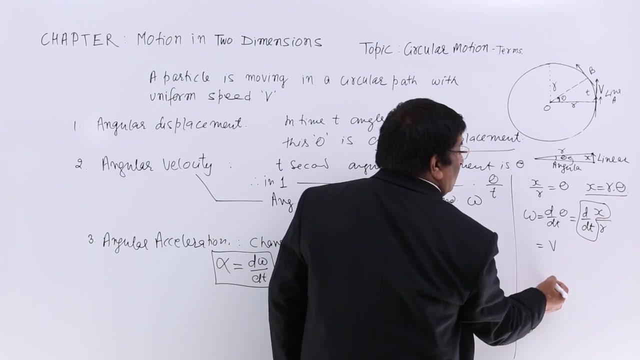 we can say: x is equal to r theta. Linear displacement is equal to angular displacement multiplied by radius. Again, what is omega? Omega is equal to d by dt of theta. So this is equal to d by dt of theta, is equal to x upon r dx by dt. this dx by dt is equal to V divided. 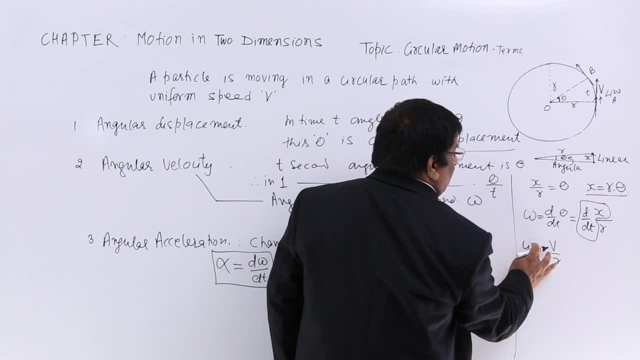 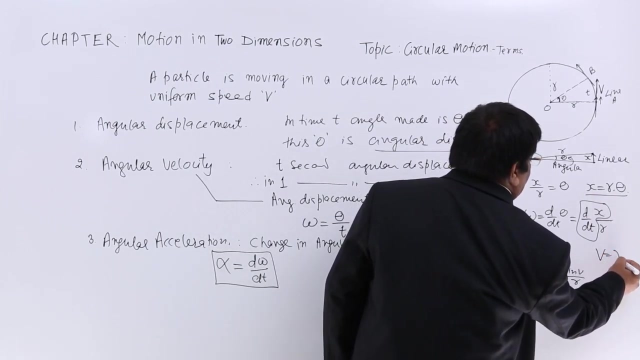 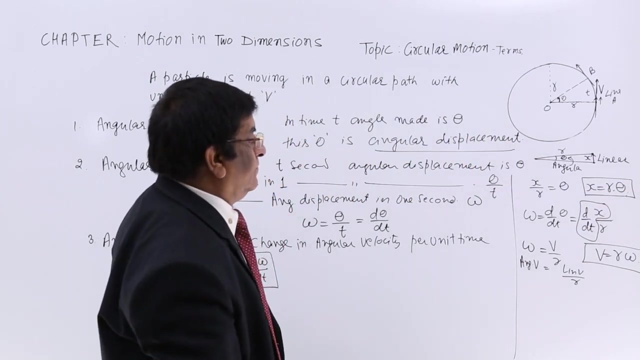 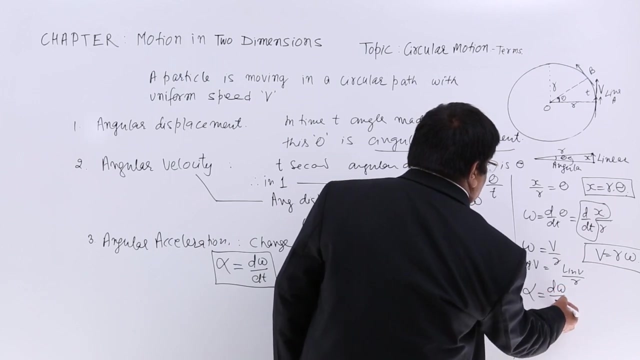 by r. So omega is equal to omega. is what Angular velocity is equal to linear velocity divided by r? or we can say: V is equal to r omega. Then come to third alpha, that is angular acceleration. This is d omega. So that is d omega by dt, d by dt of omega. and omega is equal to V upon r, V upon r. Now, 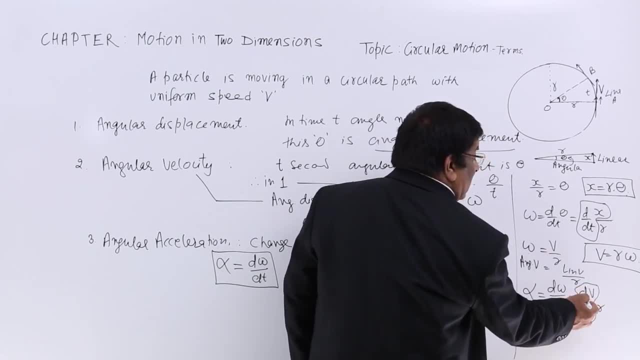 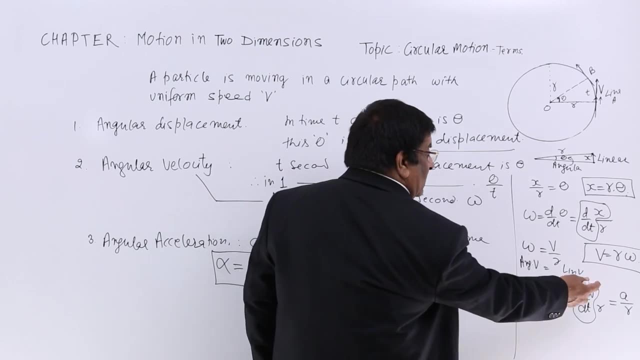 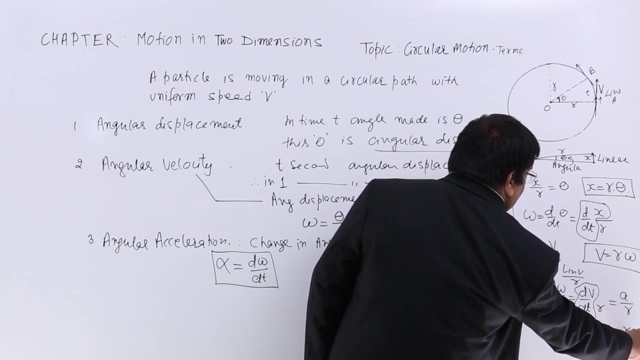 dv upon dt is linear acceleration. So we can write it linear acceleration. a divided by r, So alpha is equal to a upon r, So a is equal to r into alpha. So dv by dt is linear acceleration. Okay, 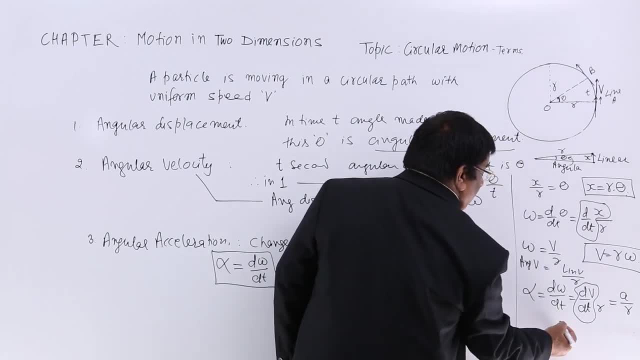 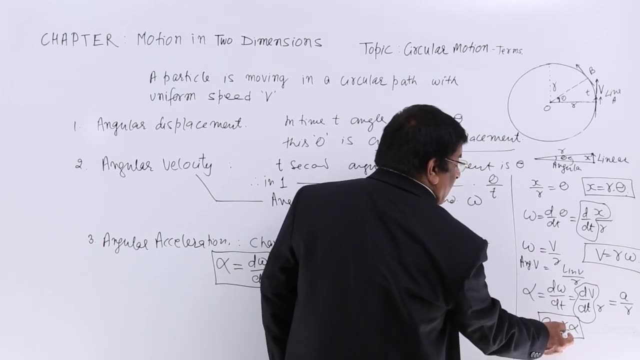 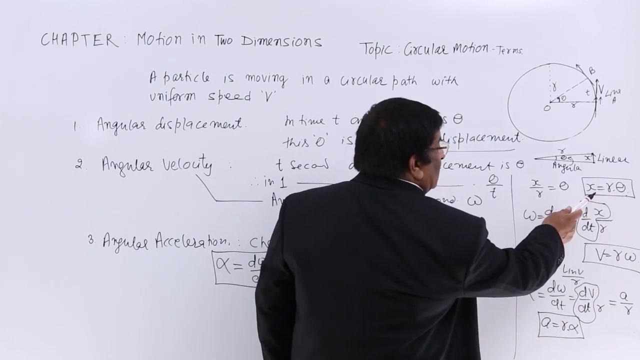 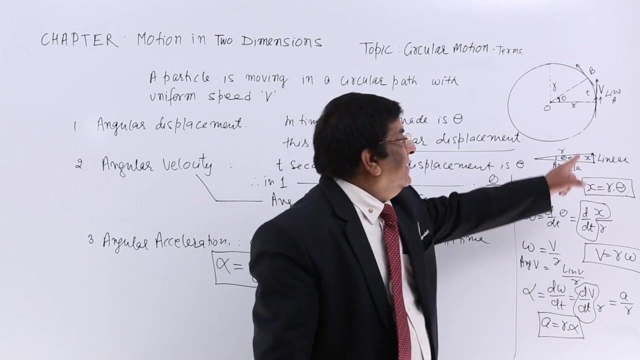 Okay, Thank you very much. Thank you, Thank you. A is equal to R into alpha and what is A? Linear is equal to: radius into angular acceleration, Linear velocity: radius into angular velocity. Linear displacement: radius into angular displacement. So please remember this relation between linear characteristic of this point to the angular. 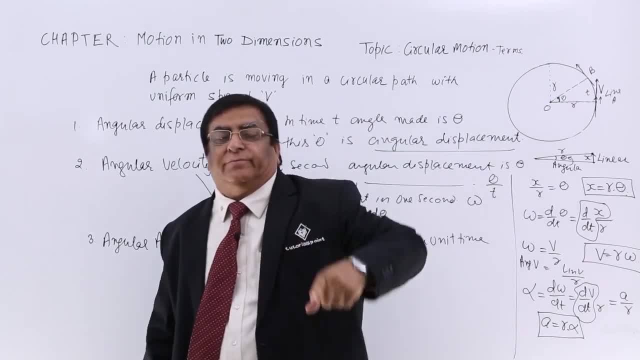 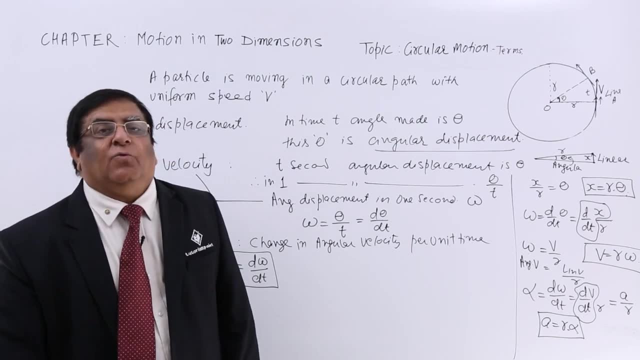 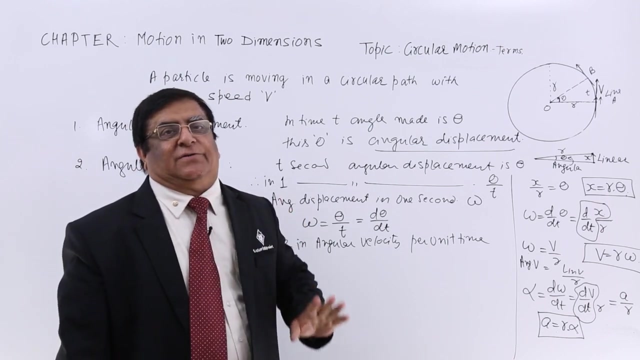 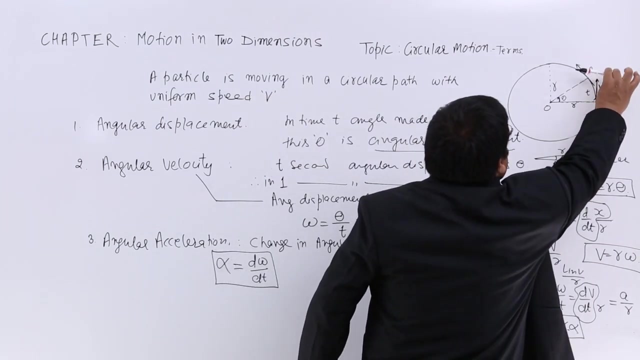 characteristic which is happening here Now: linear velocity, displacement and acceleration are vector quantity. What about angular displacement, velocity and acceleration? Answer: these are also vector quantities. If these are vector quantities, then what is this direction? It is this direction or this, or this or this? Answer: no, 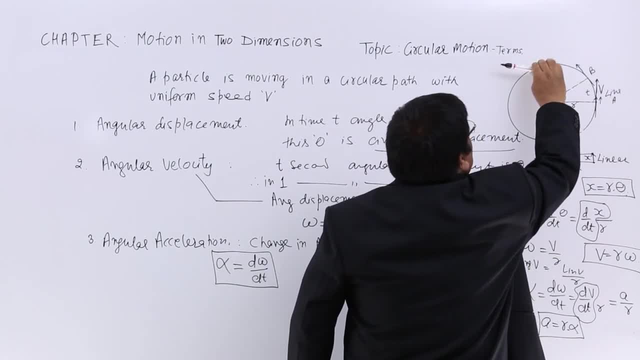 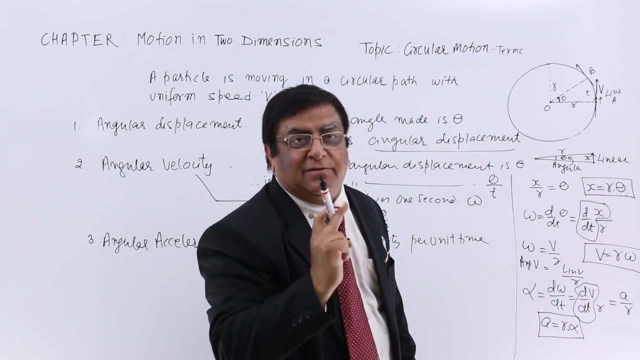 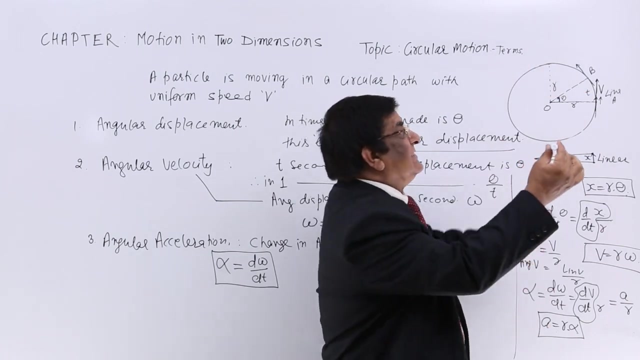 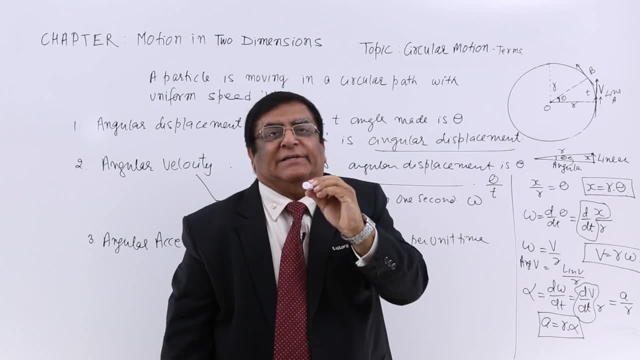 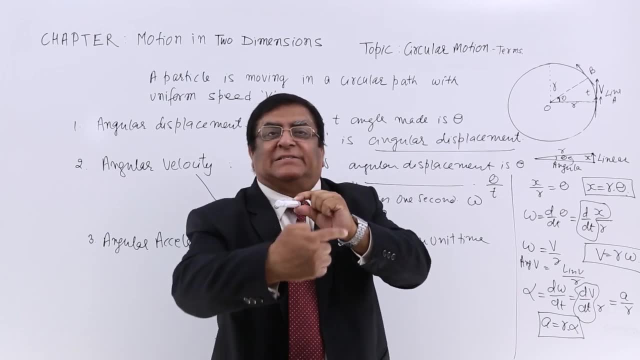 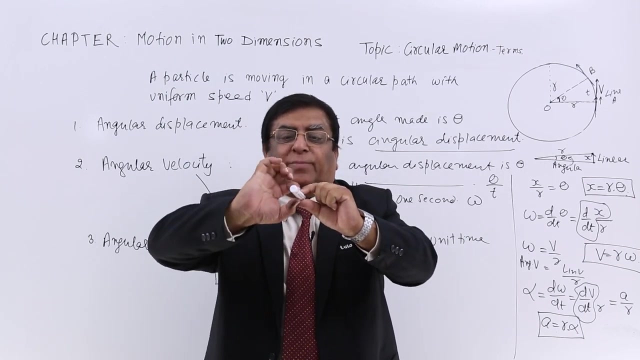 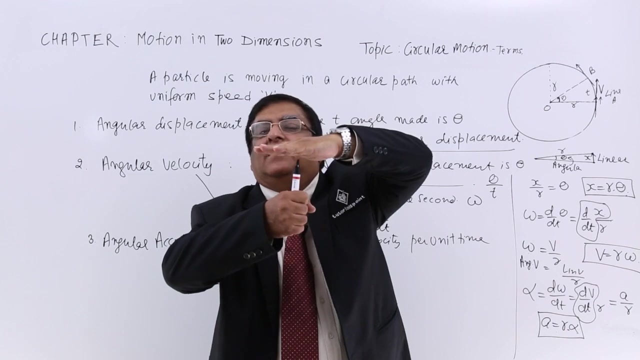 it. The direction of all angular quantities are taken along this axis. The direction of circular motion is taken along this axis because the direction of this circle is controlled by this axis. Have you seen umbrella circle? If I tell you, please change the direction. 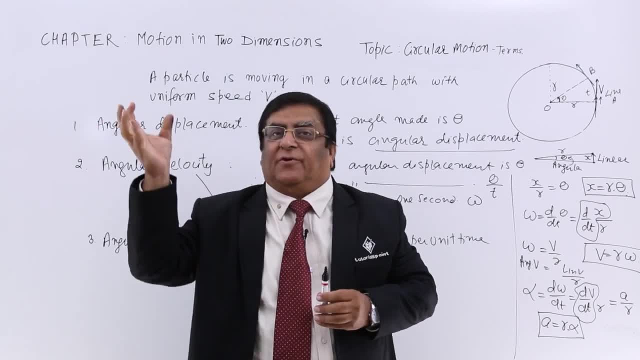 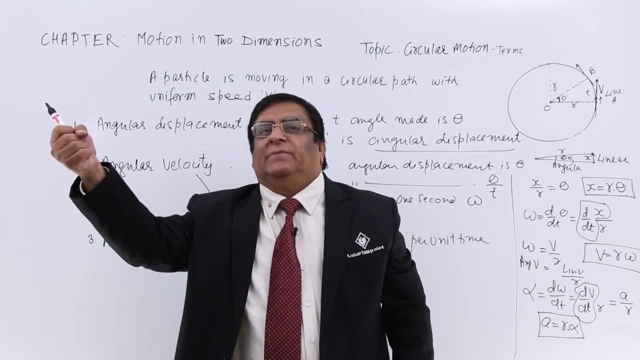 of umbrella, put it on this side, because the rain is coming from this side. What you will do? You will not touch the umbrella. You will handle the axis and put it here. This is the direction. Who controls the direction Axis? If I ask you, please put this umbrella on. 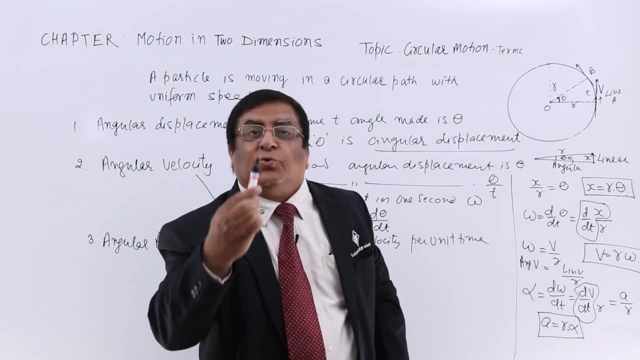 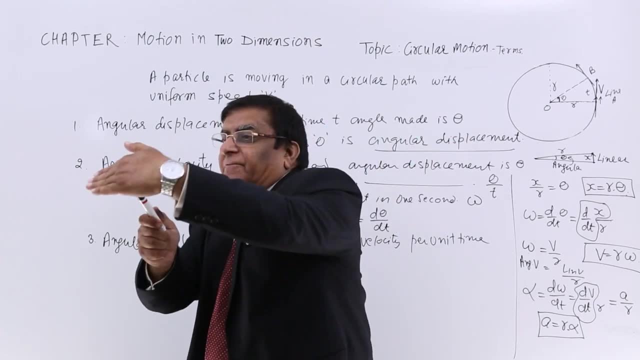 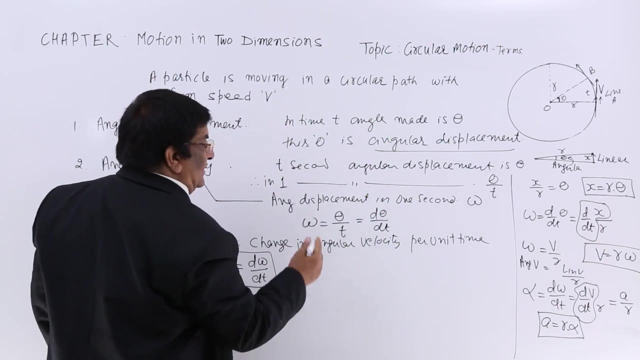 this side, This handle you will direct on this side. So who controls the direction of a circle? Its axis This way, this way, everywhere, you are changing the direction of the circle. So please remember, all angular quantities have a direction along axis This, This, This. 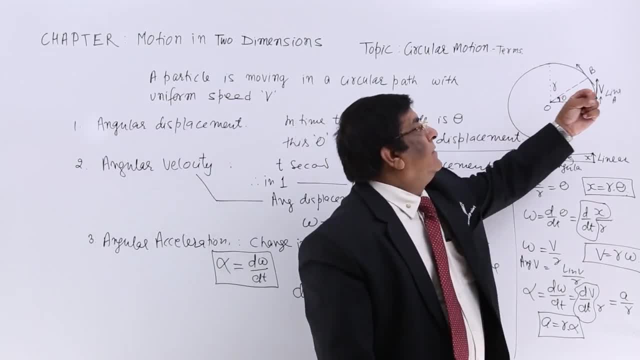 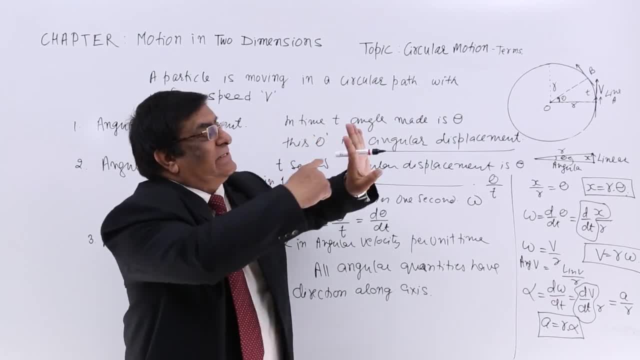 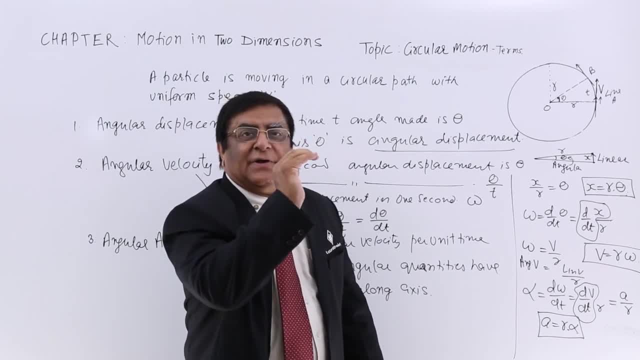 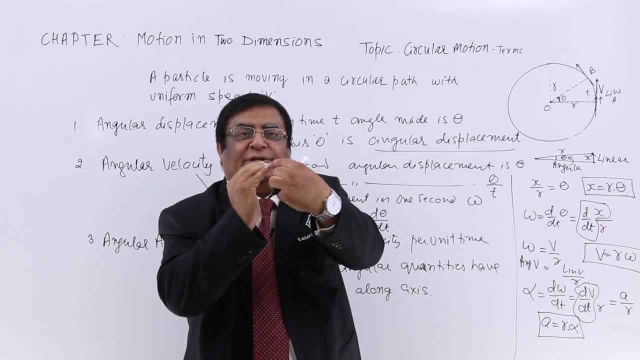 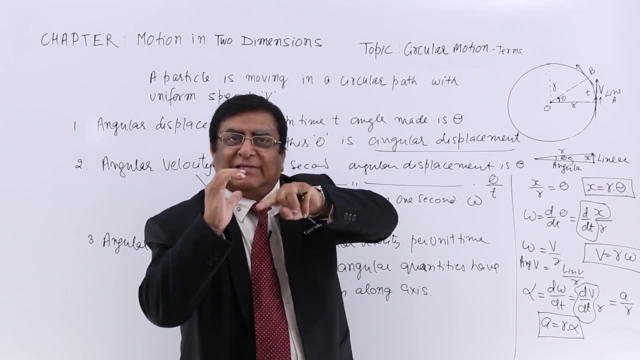 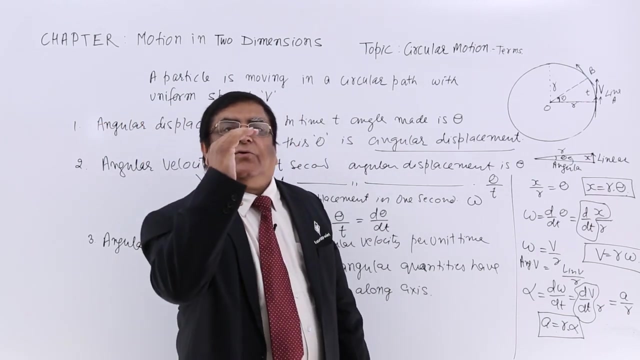 the fingers and this is the direction of rotation. If something is rotating like this, put it like this: If something is rotating like this, that is anti-clockwise, then you put it like this: Now, when you place the fingers along the rotation of the particle: 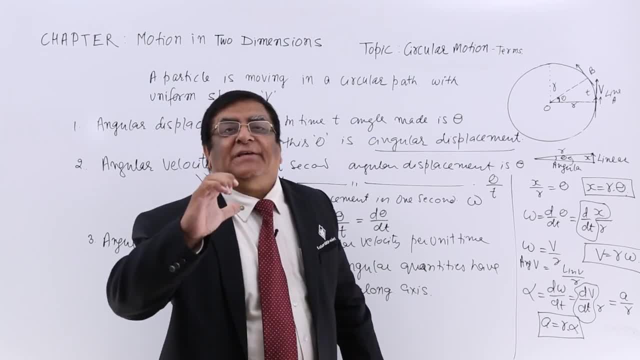 then your thumb is always giving the direction of rotation. Well then, what you have to do is you have to follow the equation from the second. Ok, That is why, when you have a number, if you have only one number in your future life, 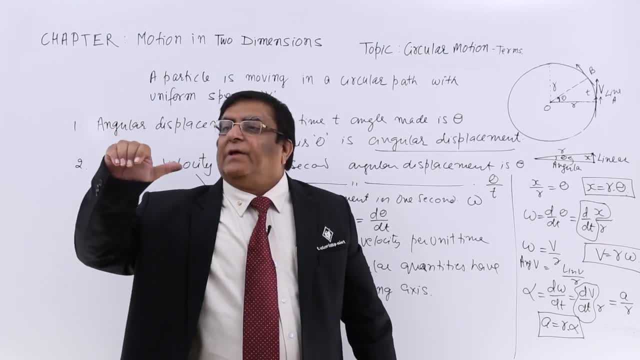 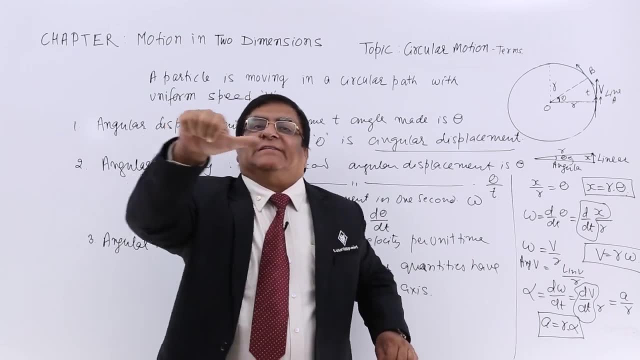 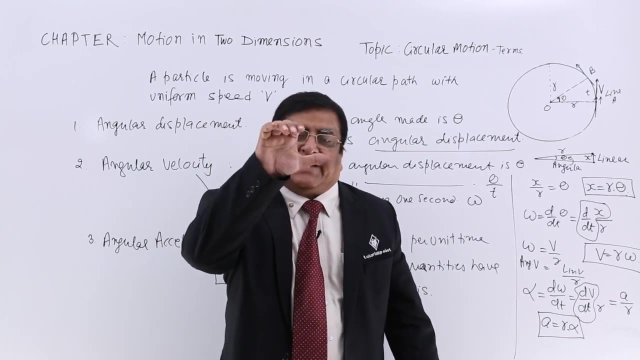 and when you have a value of whatever being equal to zero and whatever is greater than motion, circular motion. If particle is moving like this, this is the axis, this is the direction of angular displacement, angular velocity, angular acceleration. And if the particle 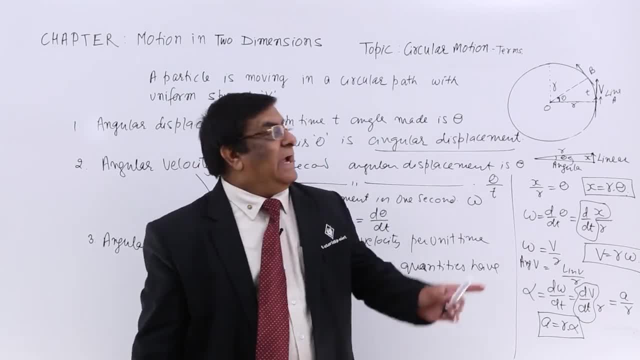 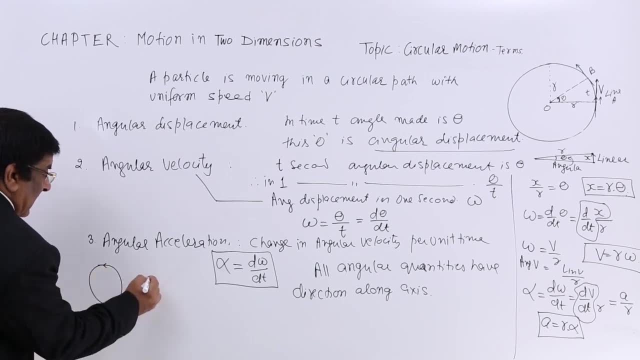 is moving like this. this is the direction And with this we can decide what. if a particle is moving this way and a particle is moving this way, Then here it is coming out, For coming out, we make a sign. dot. Here it is going in, For going in, we will make a sign. 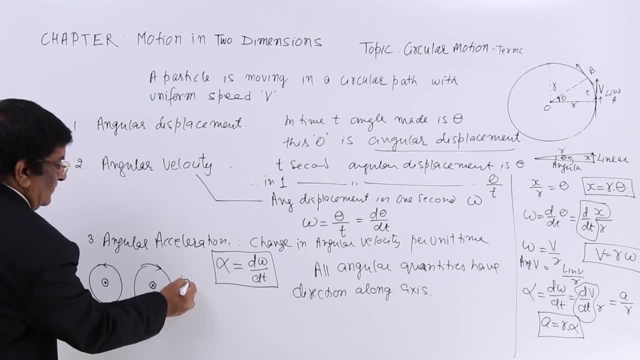 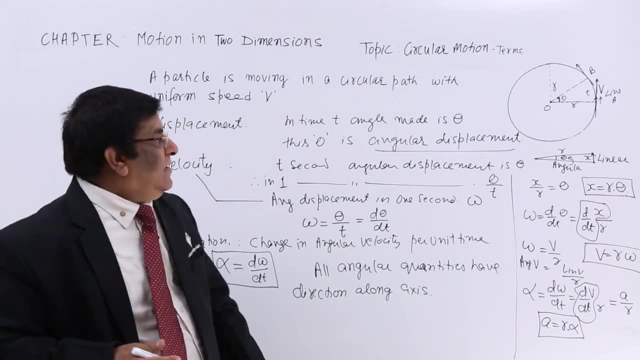 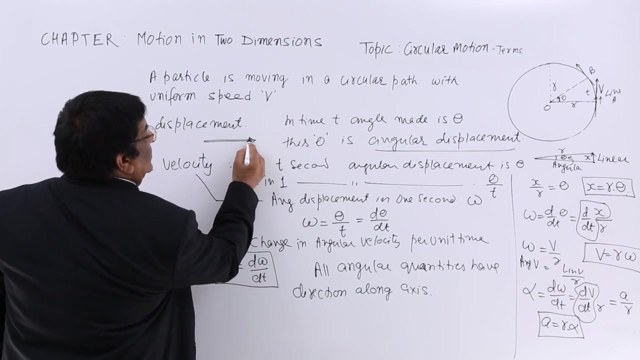 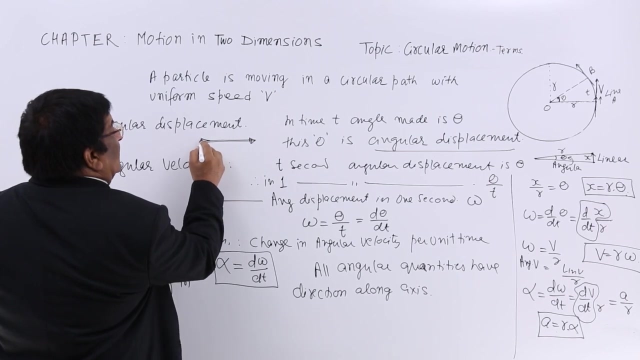 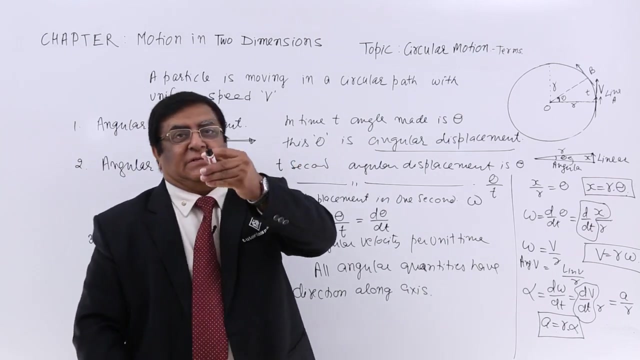 cross in here out, You must have seen an arrow. If you have seen an arrow, this, a good arrow, has this In the front and in the back it has got a feather like this: Here is a cross If the arrow is coming towards you see this. 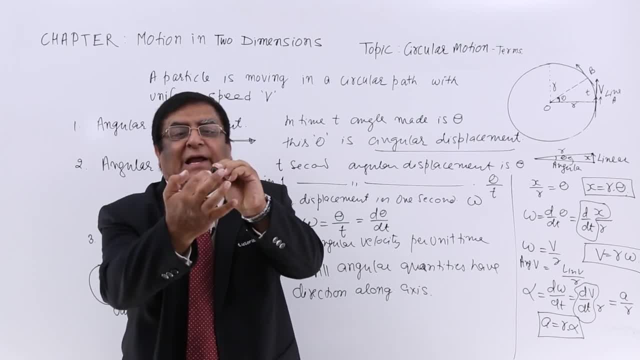 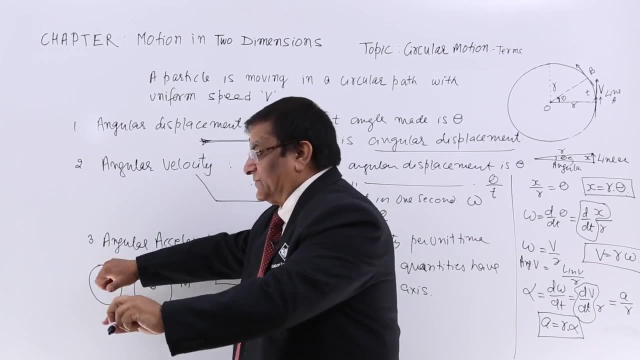 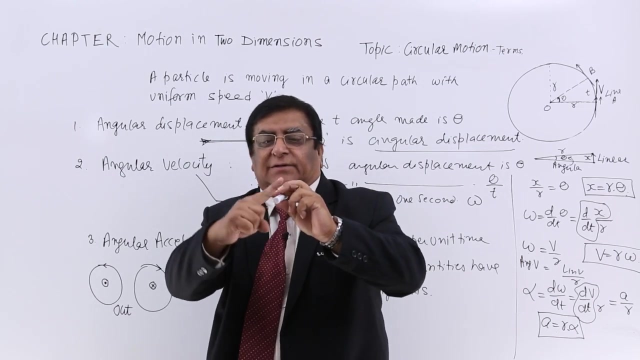 This is coming towards you. What do you see? A circle and a dot towards you. Okay, This, This is coming towards you. This is coming towards you. But if an arrow goes here, what do you see here? Feather, The two feathers are like this, in a cross manner. That is this. 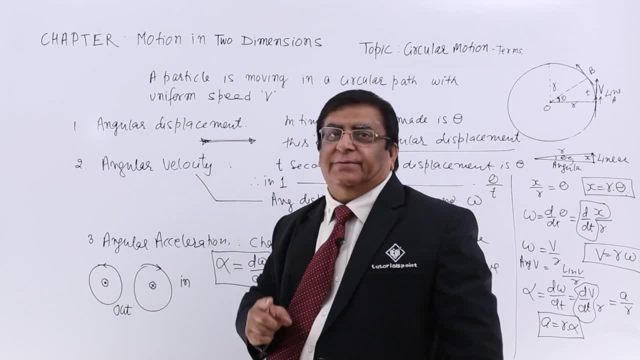 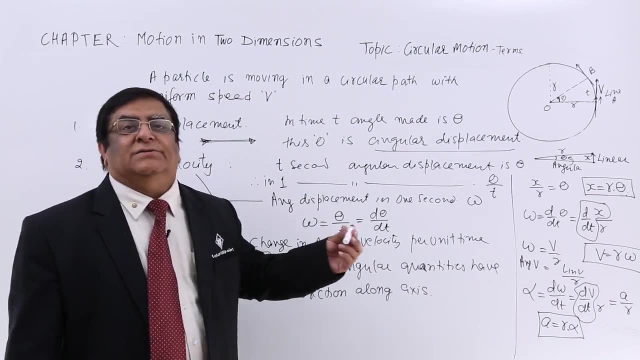 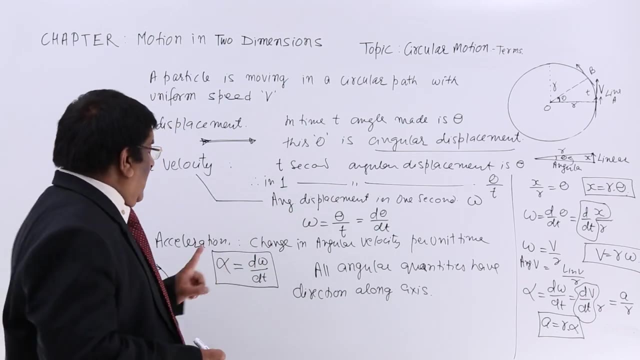 So this is going inside, This is coming outside. Okay, This is done. So this is direction of the all circular quantities. But again, do they have a sign? Answer: yes, They have sign also, Out of these two motion, one is positive and one. 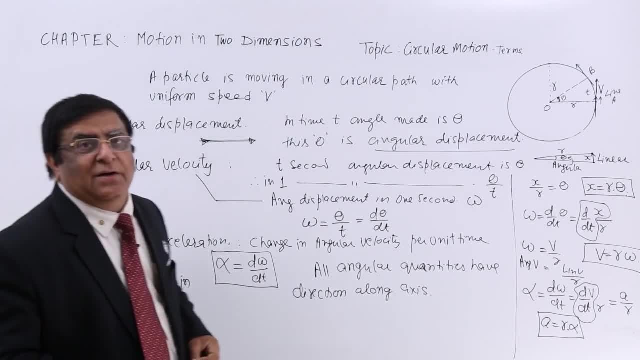 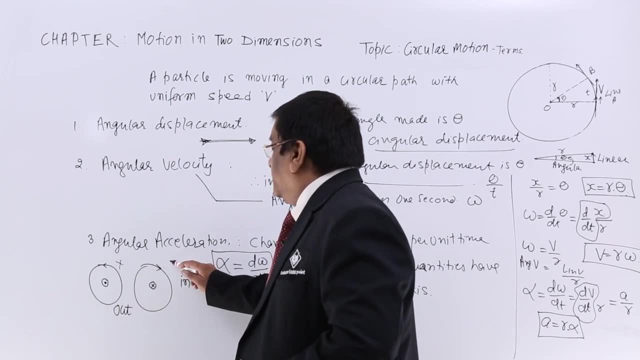 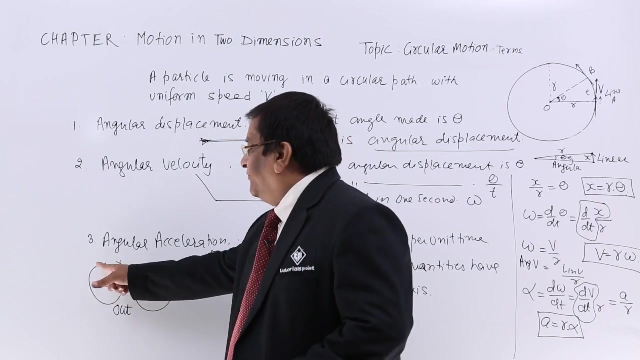 is negative circular motion, And remember the one which is anticlockwise. this, this is known as positive and this is shown as negative motion. If this is the direction of circular quantity, then this is positive and this is negative. Going inside, So this: 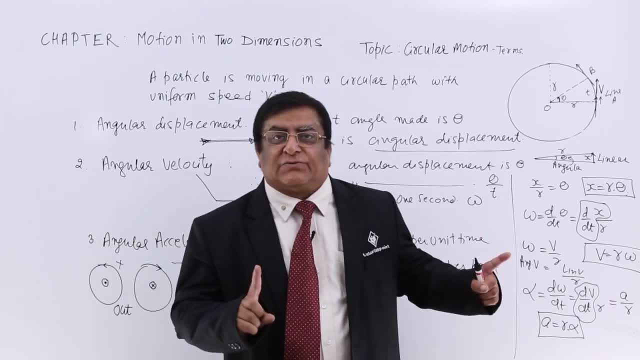 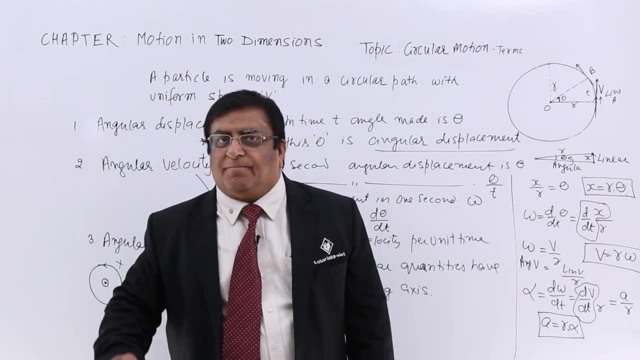 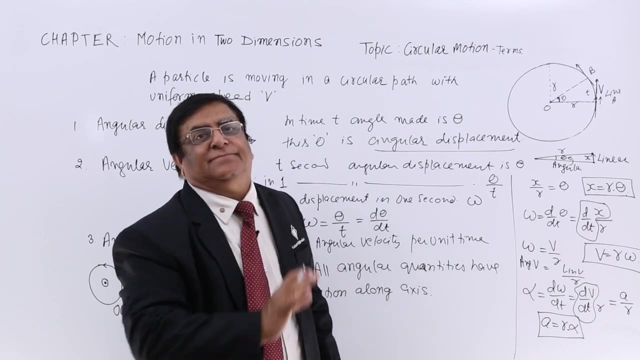 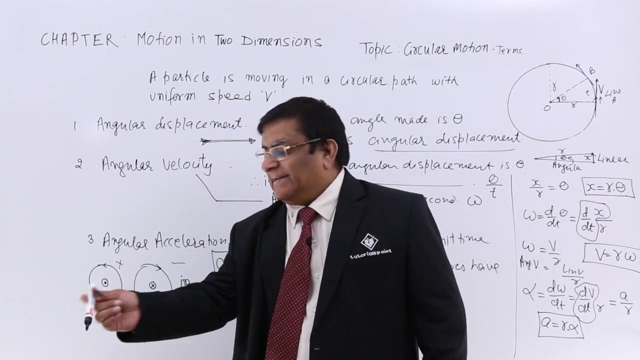 is negative. going inside X coordinate, Y coordinate, Z coordinate, This is X coordinate positive, negative, Y positive negative, Z positive, negative. So this quantity is positive Z axis, negative Z axis. So in this what you have, 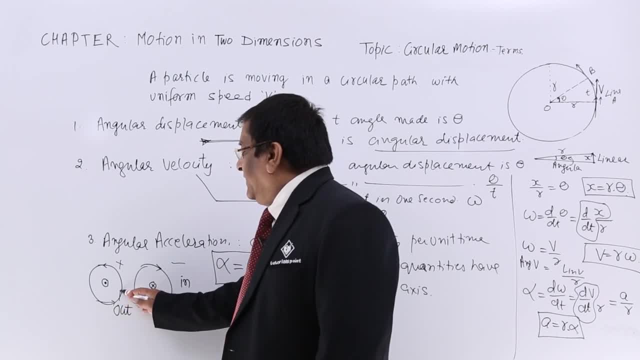 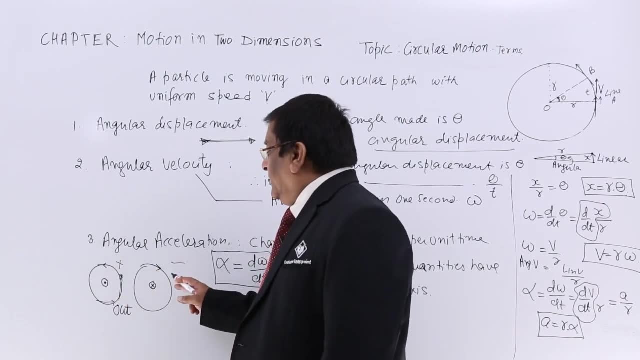 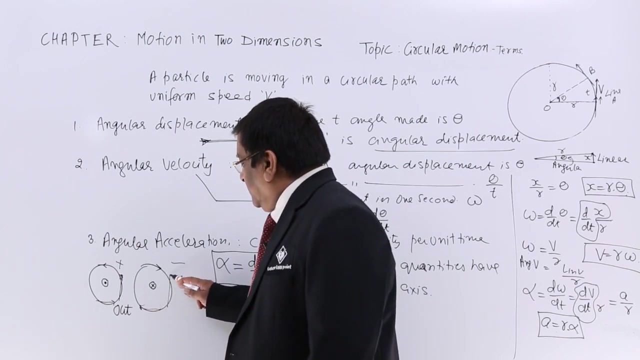 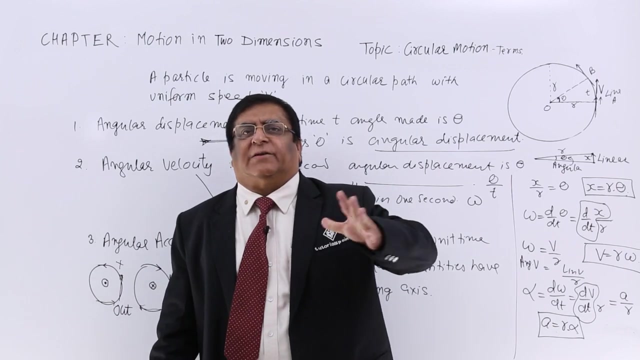 X positive, Y positive, Therefore Z positive. So this is a positive motion. Here you have this: X negative and Y negative, Y X. this is negative, But this can be explained. when we will come for vector product There we will see it thoroughly, Otherwise now you 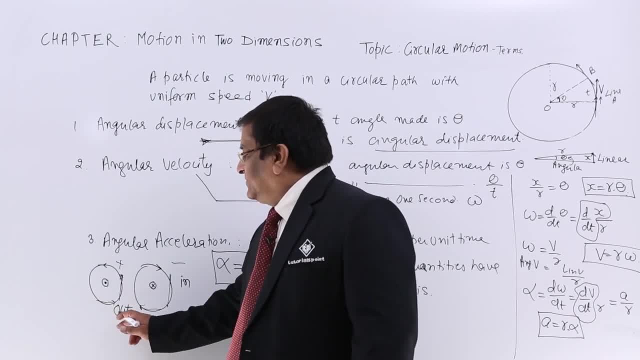 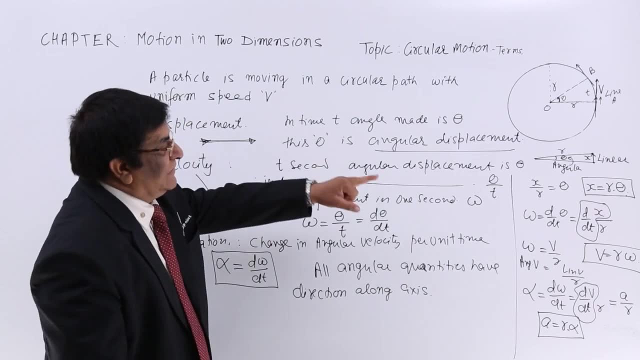 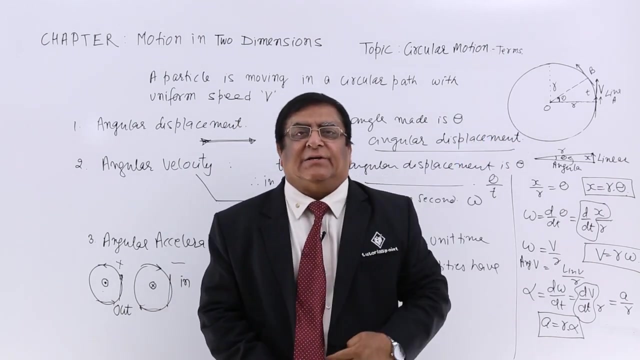 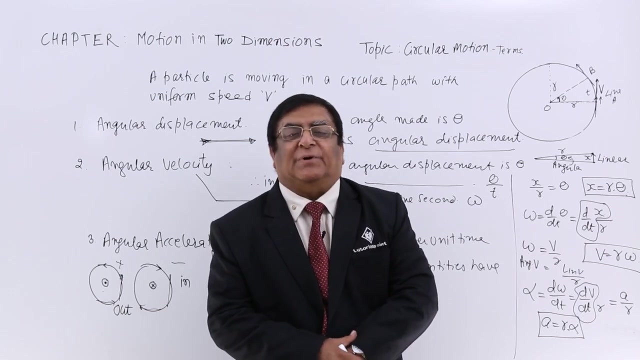 always remember that anti-clock is positive, clockwise is negative. So these are the equations, these are the fundamental terms in circular motion. In the next lecture we will find out what is the acceleration, which is known as centripetal acceleration, which makes a 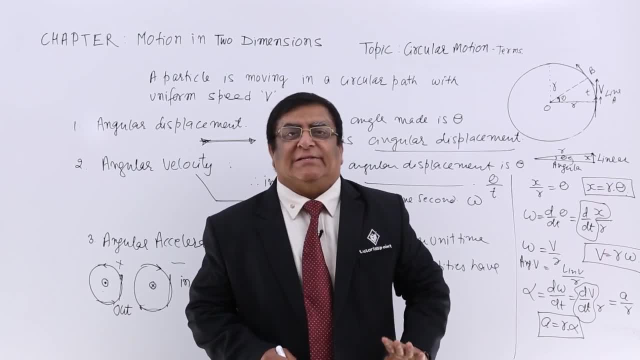 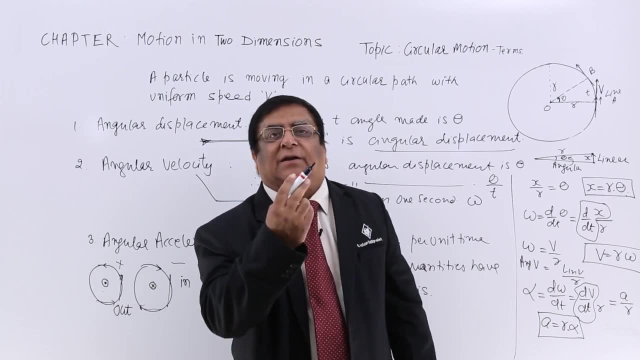 particle to make a circular motion, Otherwise every particle which is going straight. why it should make a circle. And when it is making a circle, what is meant by a centripetal acceleration? Thank you.